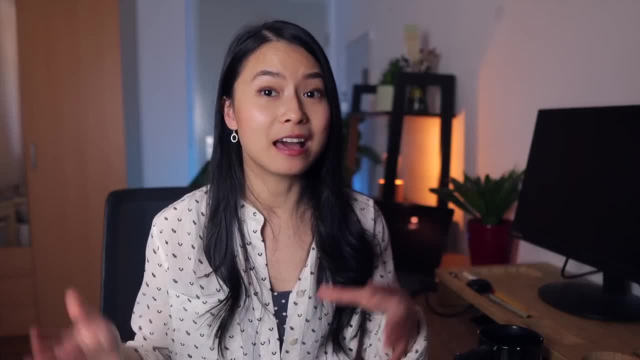 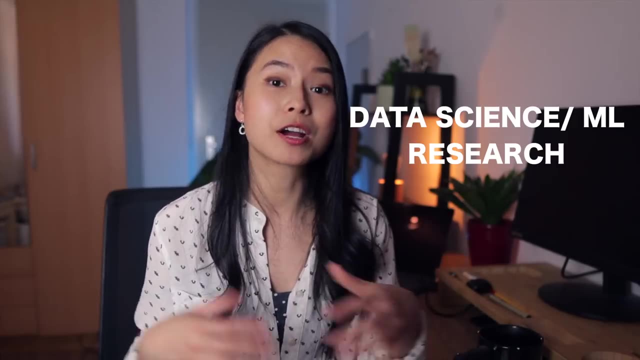 I want to make a small note here. It's important to know that the level of math knowledge you need to know very much depends on your goal. If you want to do a PhD in data science or go into machine learning research, then it's necessary to study math very well. 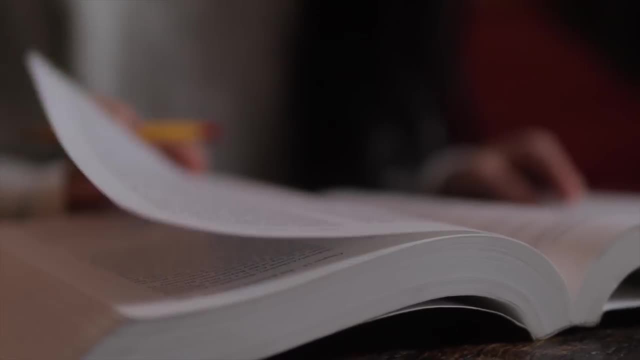 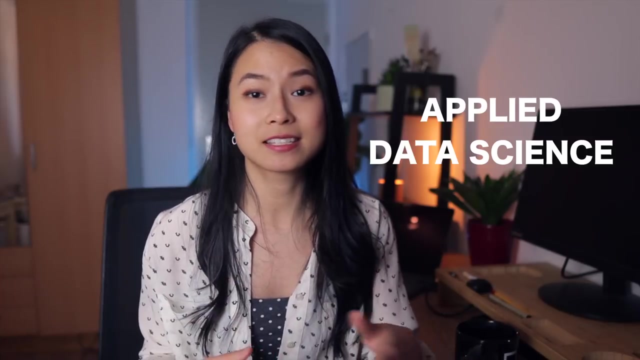 Then maybe you should grab the biggest books you can find on calculus and linear algebra and start grinding. However, I think many of us, myself included, are doing applied data science instead of doing research, meaning we want to solve business problems through data science. 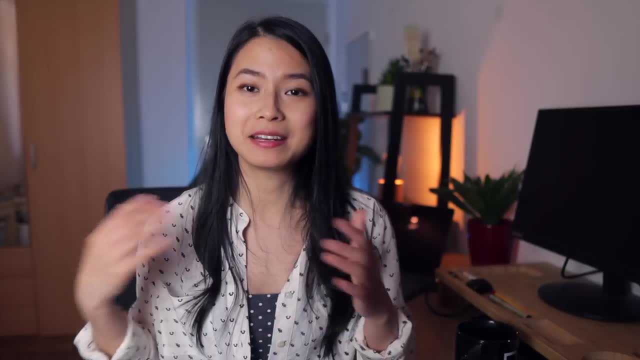 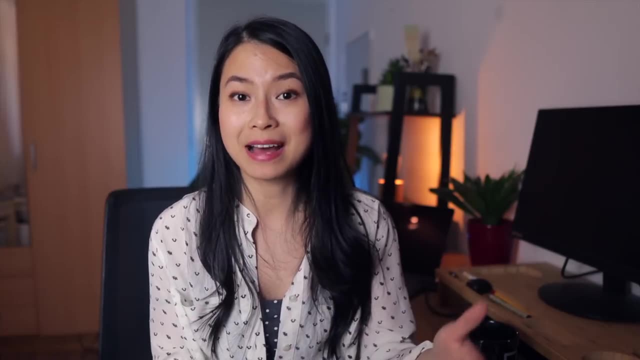 but we are not necessarily the people who study and come up with new machine learning algorithms, for example, So we might not need to know every little detail or understand the most advanced math concepts. It is okay to have some solid, high-level and basic understanding. 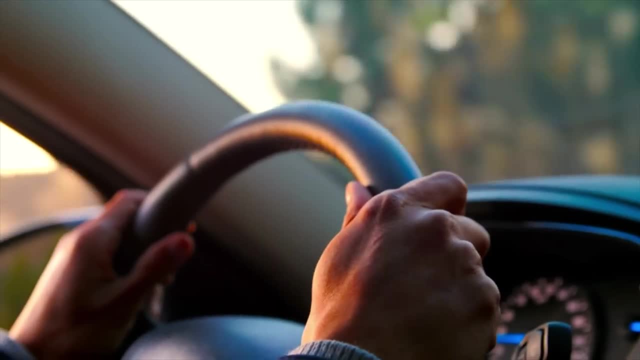 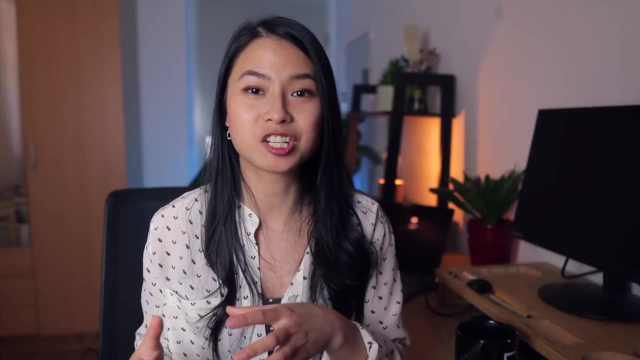 and that's probably enough. Just like when we drive a car, we care about how to drive them properly and get to the destination rather than understanding how every small component in the car engine works. You certainly can if you're a hobbyist, but you don't need to. 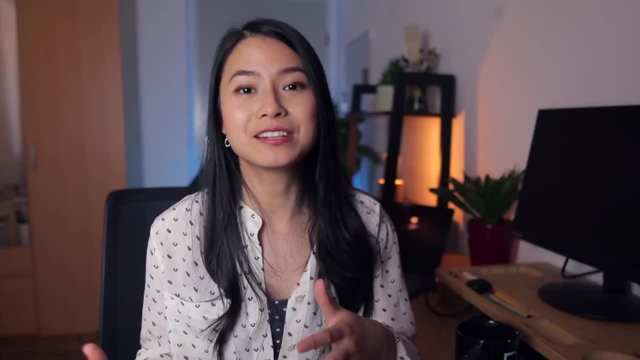 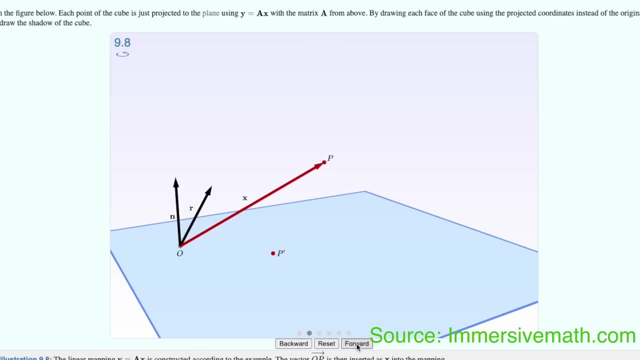 That's why not everything we're going to talk about is applicable to you, and you need to decide if you want to put them into your learning curriculum. Alright, so the first important kind of math used in data science is linear algebra. It is a branch of mathematics that has everything. 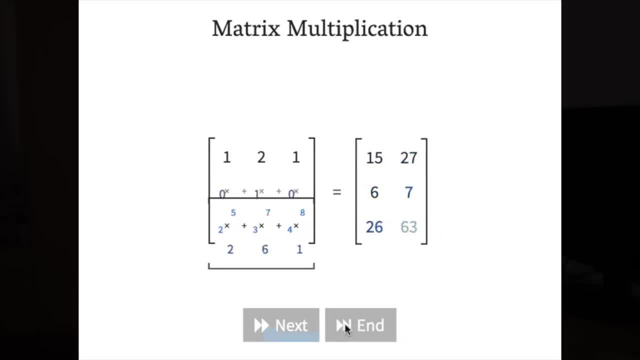 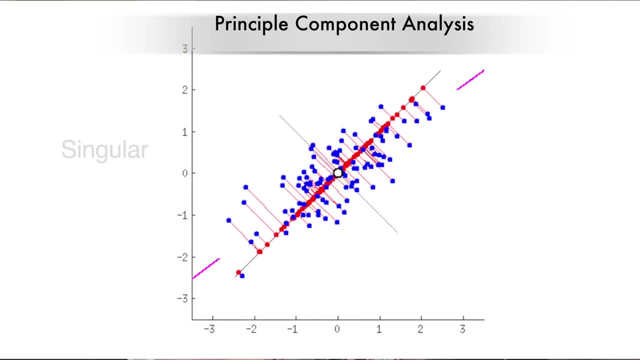 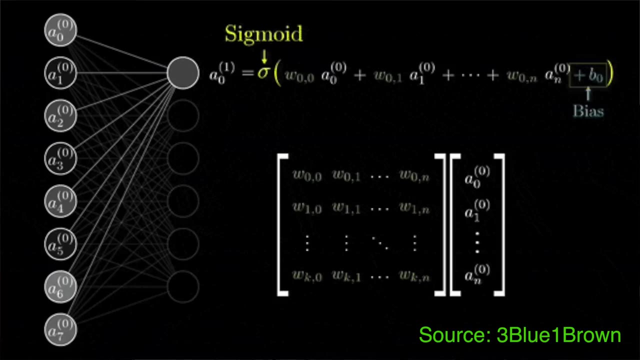 to do with vectors and matrices and the operations on them. You might encounter linear algebra in several machine learning algorithms. For example, principal component analysis uses singular value decomposition to present your data in fewer dimensions. Linear algebra is also the backbone of the calculations behind all neural network algorithms, so it is a very useful area of. 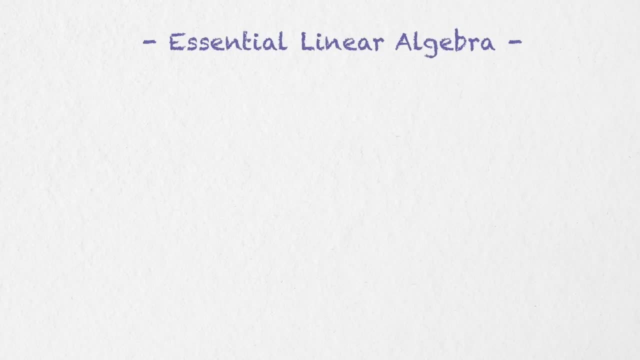 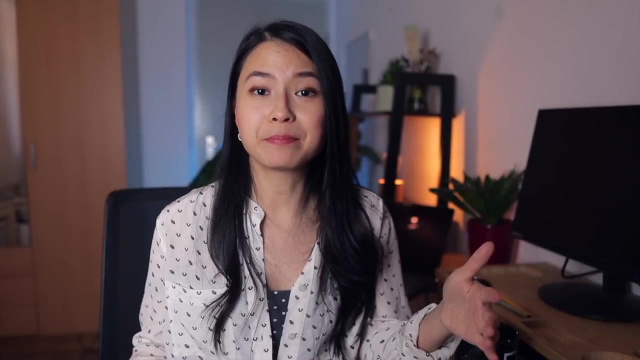 knowledge to have a solid understanding of. So let's get started. Some main concepts to know in this area is, for example, dot, product matrix, multiplication matrix, factorization, eigenvectors and eigenvalues, singular value, decomposition, and so on- The second branch of mathematics that's extremely useful for data science. 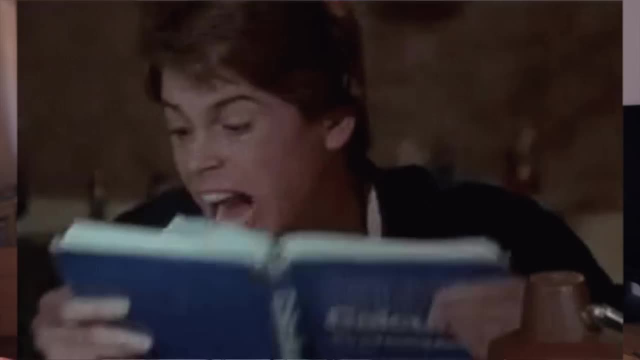 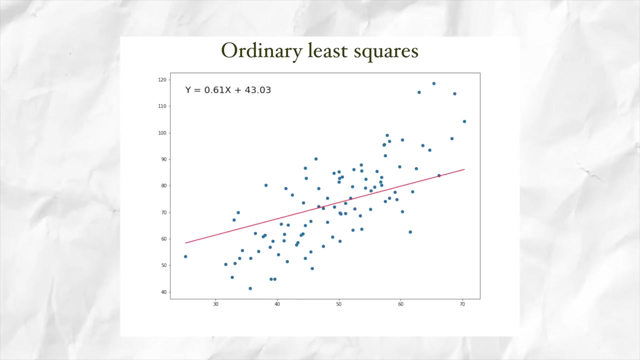 is calculus. It is the study of continuous change. Whether you laughed or hated it in college, calculus pops up in several places in data science and machine learning. If you've learned about ordinary least squares problem in linear regression or learned about the back propagation algorithm, 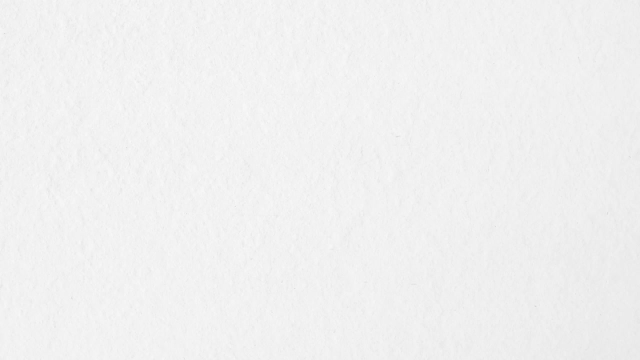 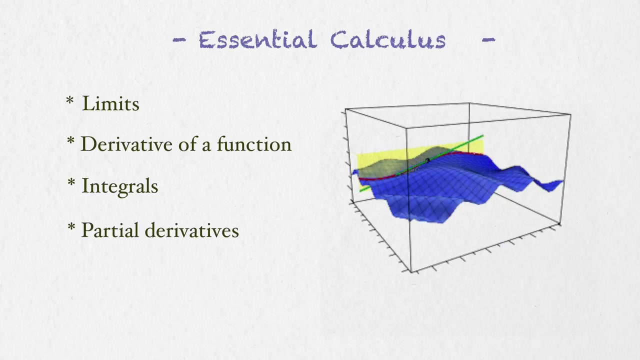 in neural networks, you might have encountered a lot of calculus. Important topics in calculus are the limits, the derivative of a function, integrals and partial derivatives and the chain rule. I used to like calculus a lot back in high school time and I actually found it quite. 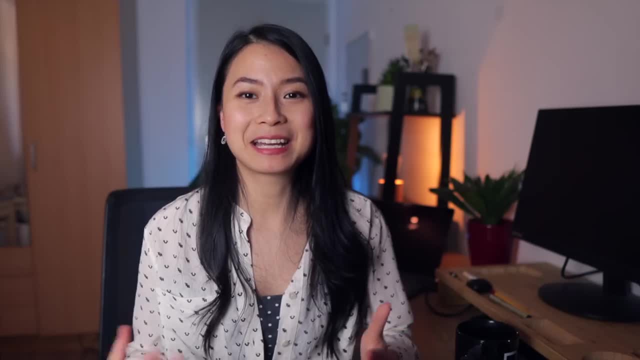 intuitive, but the more you dig into it, the more complex it can be, and so I kind of stopped digging Now. you may have to face a lot of difficulties in this topic, but I bet you'll be able to learn it. I will be sure to give you a shout out in the comments about calculus and, of course, if you're interested. 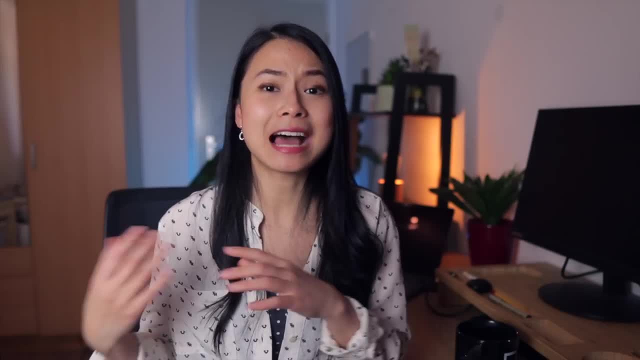 in learning calculus. you can subscribe to my channel to learn more about it and find out what you really need to know about calculus. I'll be sure to share this video with you If you're interested in learning. find that the calculus necessary for data science is actually usually not. 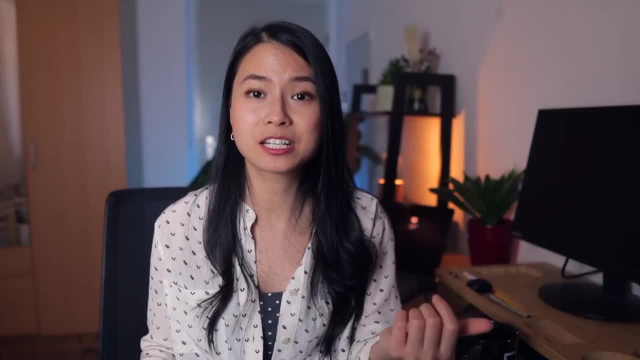 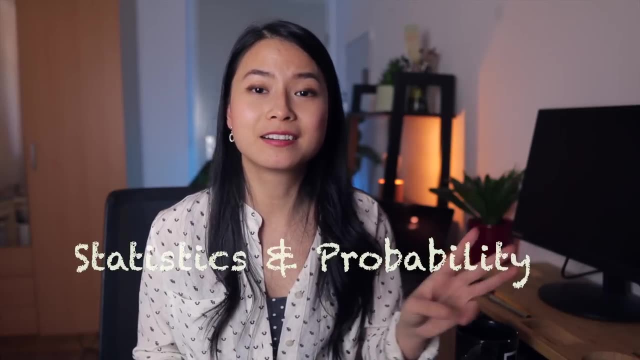 super advanced and often limited to the concepts we just mentioned, and that's good news for many of us who find calculus challenging. Statistics and probability is the third important pillar in data science. In fact, many experts in the field consider classical machine learning nothing but statistical. 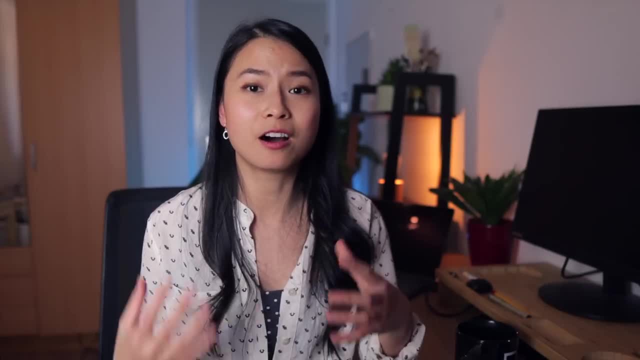 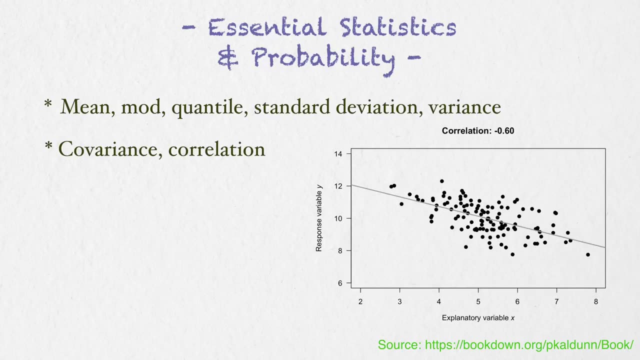 learning. Many of us are probably already familiar with a lot of basic statistics, for example the mean, mod, quantile, standard deviation, variance, covariance and correlation. Besides that, we might also encounter a conditional probability, for example when you learn about Bayes' theorem, and we should also be familiar 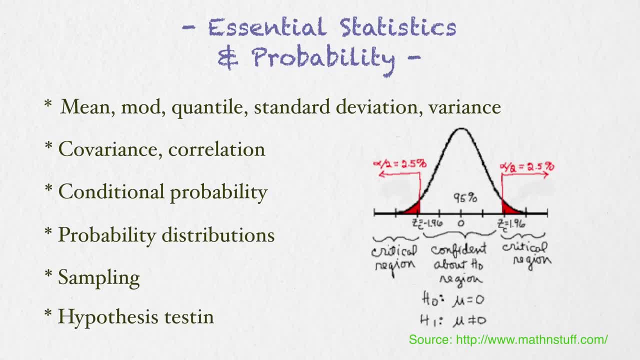 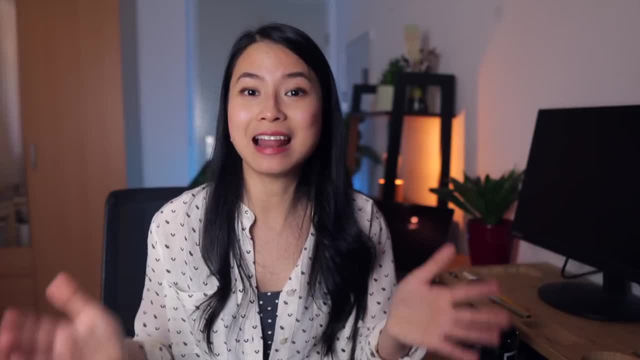 with topics such as probability distributions, sampling and hypothesis testing. Again, what you need to learn really depends on what you want to do. Honestly, I can't remember the last time I used t-test or worked with t-distribution anymore. I don't even do hypothesis. 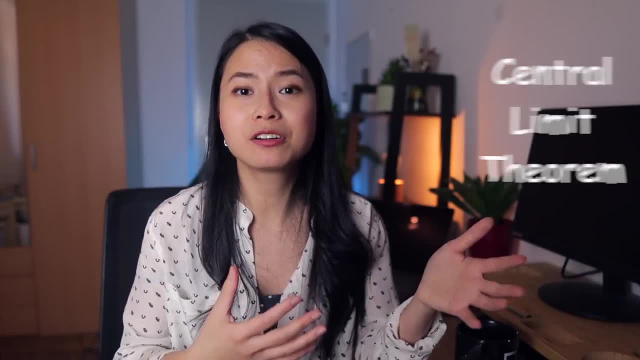 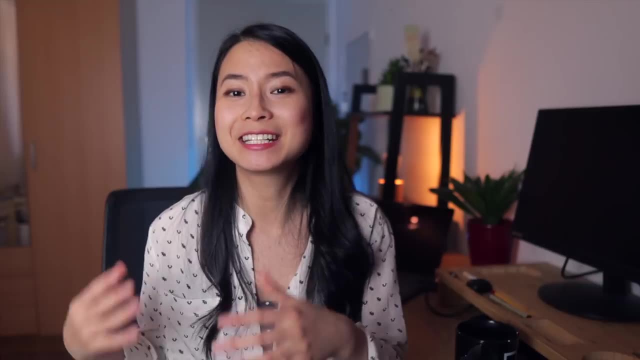 testing. I don't even do hypothesis testing. I don't even do hypothesis testing in my work. Also, many concepts, for example central limit theorems, are important in traditional statistics but are no longer important in modern data science, so probably you don't need to sweat about them. You can also find in: 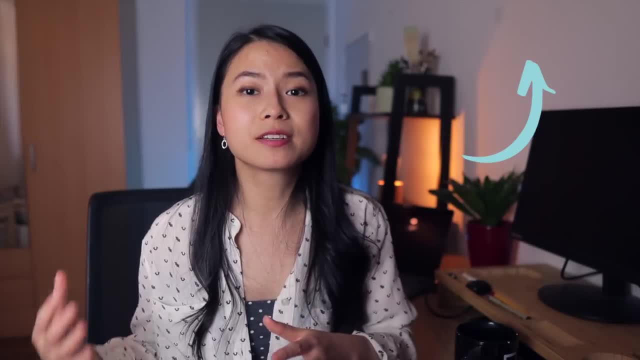 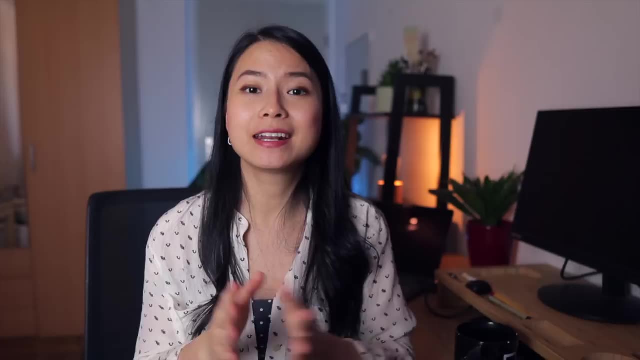 another video on my channel some detailed explanation of most of the statistical concepts you need to know for data analysis. For some of us who might be curious about computational systems, data structures and algorithms, you might want to learn a bit discrete math, but it's not strictly necessary in 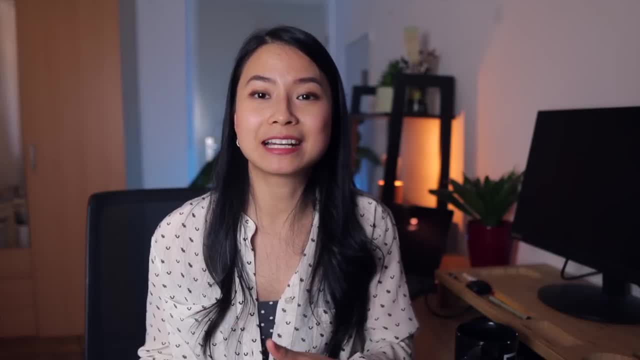 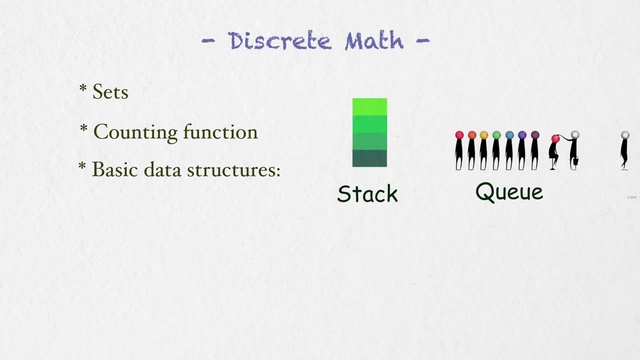 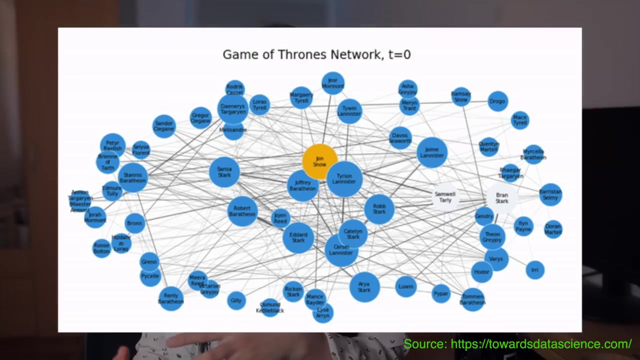 my opinion, I only learned discrete mathematics in my computer science degree and it's quite interesting to learn about sets, counting functions, basic data structures like stacks, queues, graphs, hash tables and their implementations in different programming languages. For example, if you work with social network analysis, you 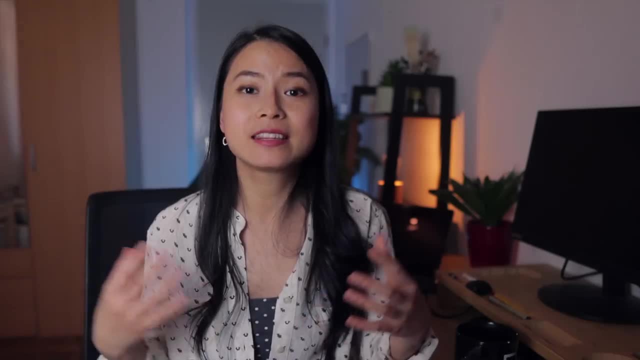 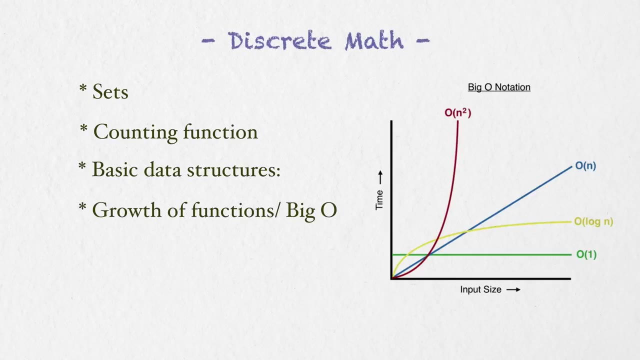 might find it useful to know about graph data structure and the algorithms you can perform on graphs. Another very useful concept you learn in discrete math is the growth of functions and the big old notation. When you have to make a choice of algorithms to use in your project, it's really useful to 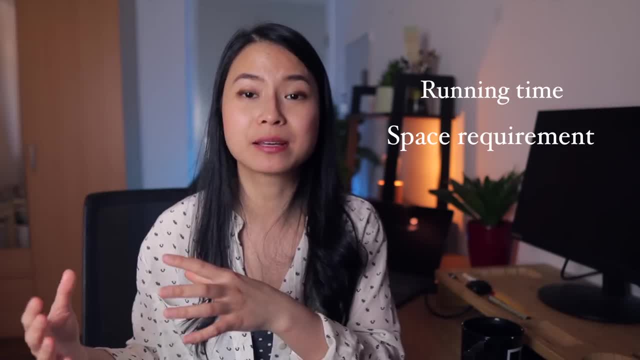 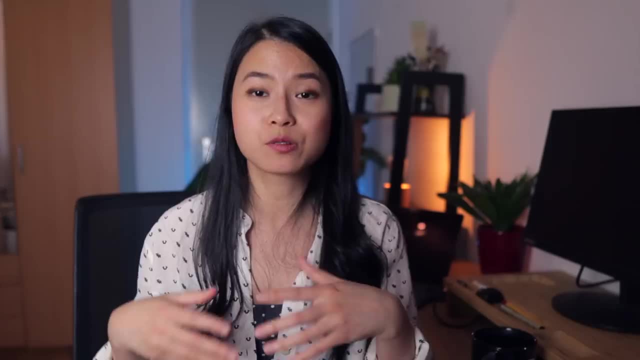 understand the running time and the space requirement of an algorithm using big old notation, But I feel like all these concepts are probably more useful further down the road for those of us who want to level up in our data science careers than for those of us who are just starting out. Okay, so it seems. 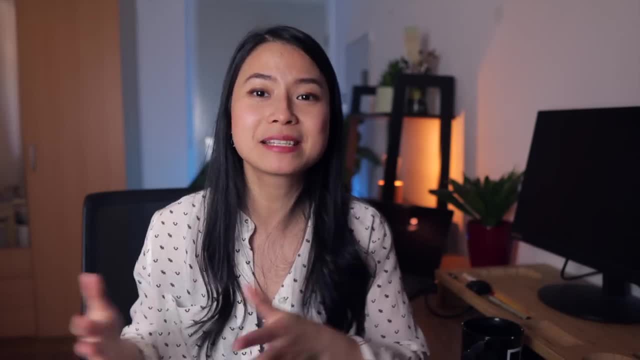 like there are tons of things to learn. Now let's move on to some of the tips that could help you learn math for data science more effectively. The first thing, as I mentioned earlier, is that there are tons of things to learn, So I'm going to share some of the tips with you in libertine, for data science. 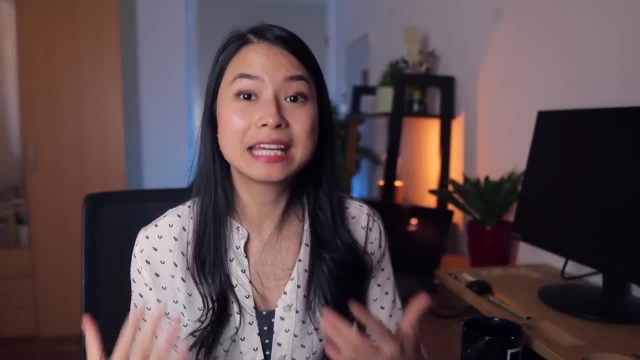 Then you can keep your mind focused on data science in the comment section below. The first thing, as I mentioned earlier, is to keep your goal in mind so that you don't unnecessarily overwhelm yourself with things you don't really need to know, For example. 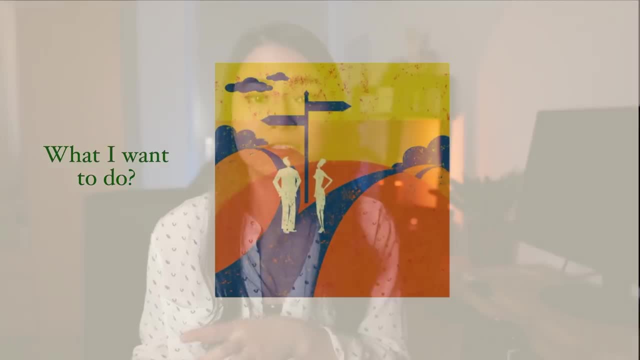 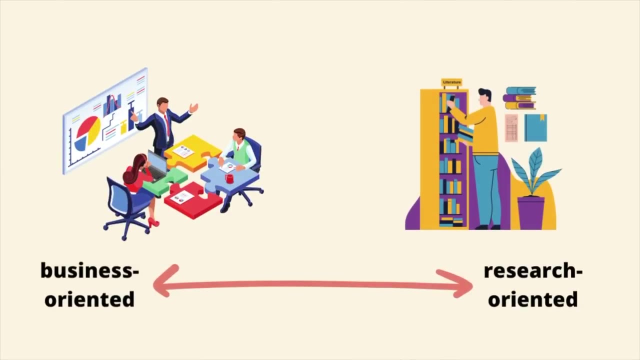 think about where you want to position yourself in the data science field. You can choose to be more in the direction of applied data science, aka more business-oriented kind of data science, or you can choose to be more in the direction of data science research, And from this, 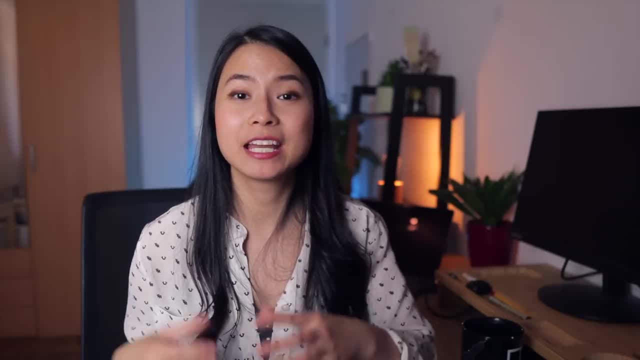 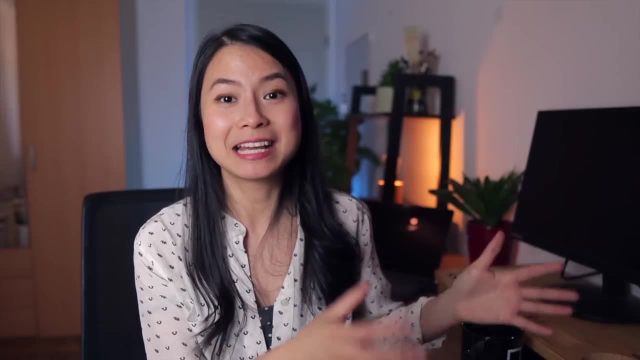 you can determine for yourself how deep you want to go into a topic, if at all. For me, I know I wouldn't want to become a data science researcher. I'm more inclined towards being an implementation person and I like to create really tangible stuff. so I usually just make sure to. 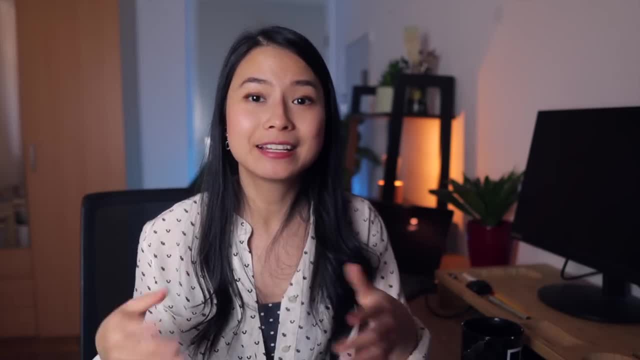 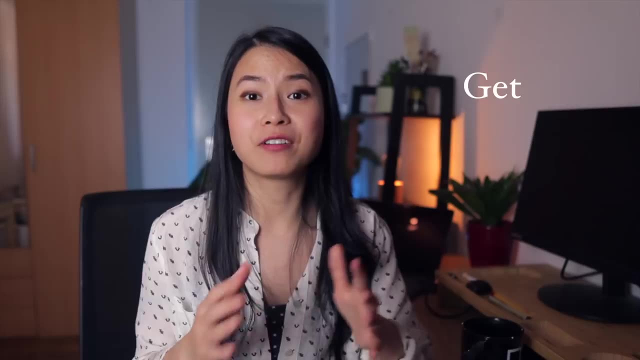 learn things well enough to be able to explain them in my own way to other people and implement them to solve a problem. The second tip that I think is relevant for everyone is to get the fundamentals right. There's really no shortcut, because everything is built on top of some. 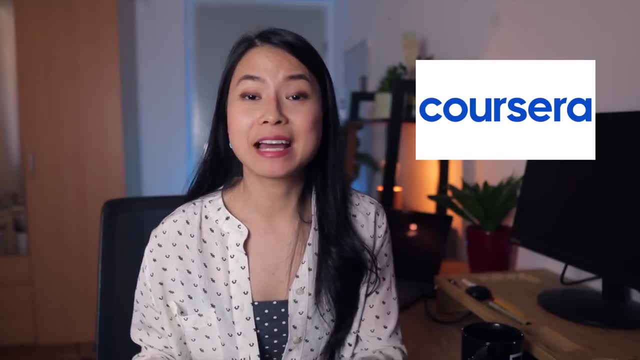 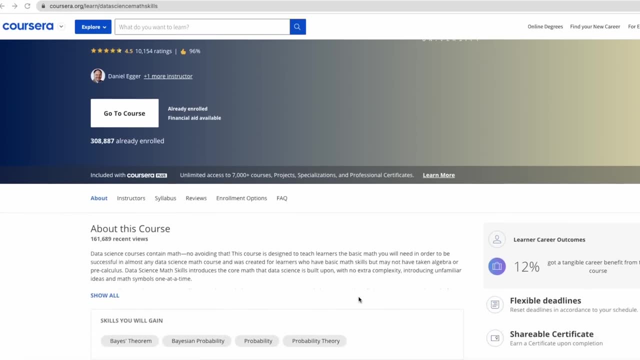 fundamental concept. If you like learning on Coursera, like me, you should definitely have a few really helpful math courses for data science. The first one is Data Science Math Skills by Duke University, which covers the basic mathematics that you need to progress to more. 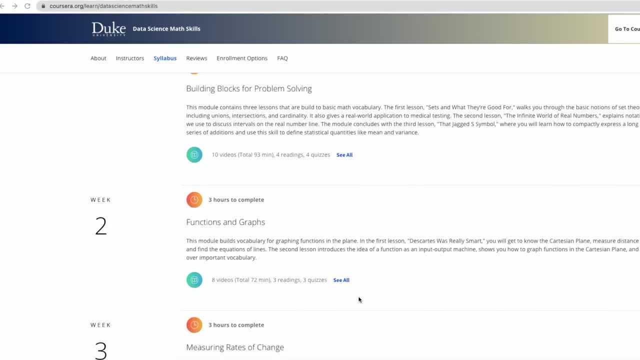 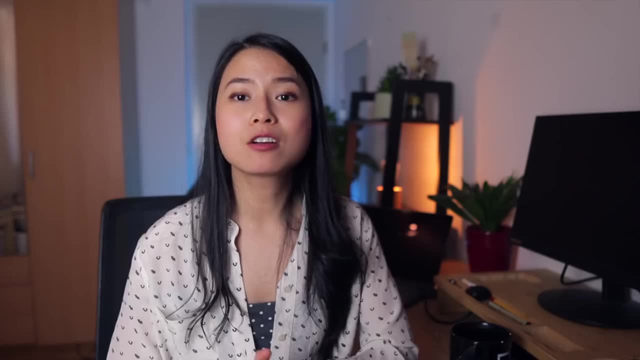 advanced math topics. So if you feel like you need to brush up your knowledge on set theory, functions and graphs, logarithms and things like that, this is a course you can start with. The second course I think is very good is the Mathematics for Machine Learning Specialization. 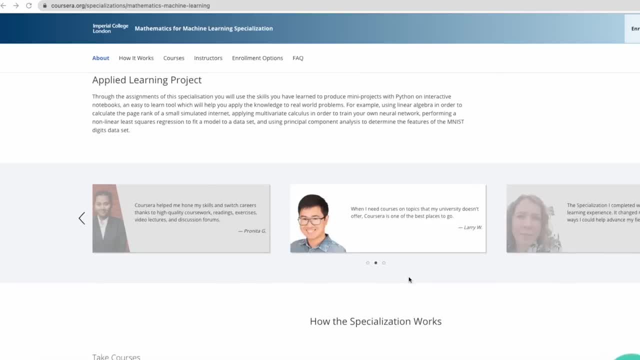 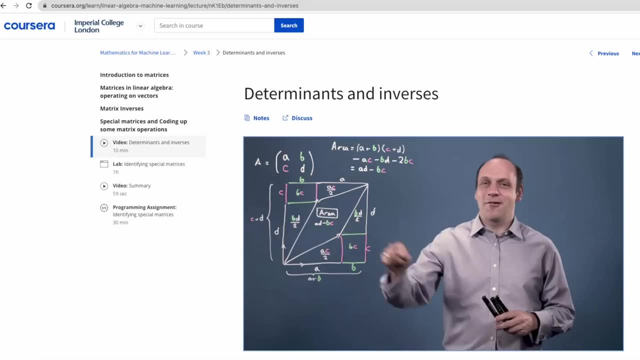 by Imperial College London. This specialization contains three courses: Linear Algebra, Multivariate Calculus and PCA, So they cover pretty much most of the math you need to learn for machine learning. It's a pity that it doesn't cover statistics, because well. 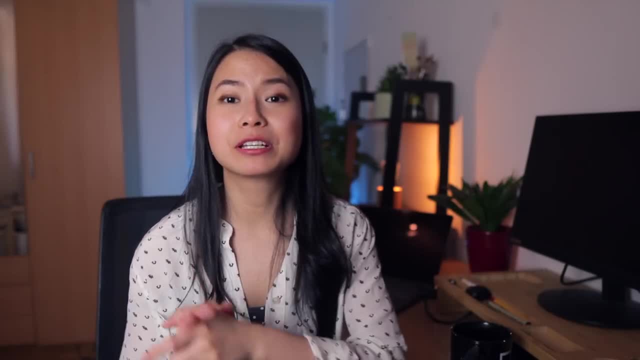 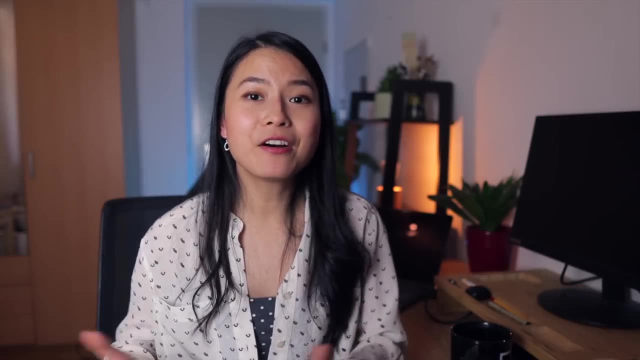 statistics is in a sense not math, But for that there are many other resources as well. In the description below I put a link to some statistics books in R that I found really helpful so you can check it out. If you know any good resources for statistics with Python, please share in the 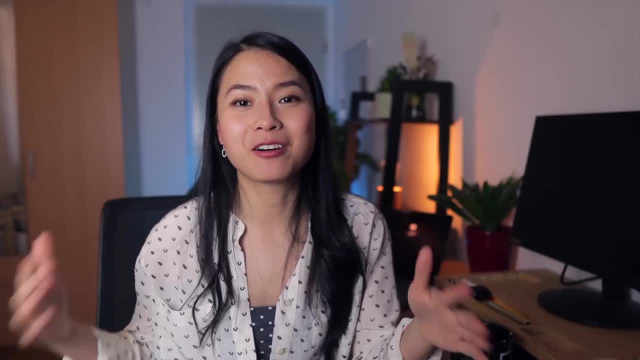 comments below. It's often easy enough to press the enroll button on an online course, but I often find that it's not as easy as it sounds. So if you're interested in learning more about statistics, please subscribe to my YouTube channel and I'll see you in the next video. Bye for now. 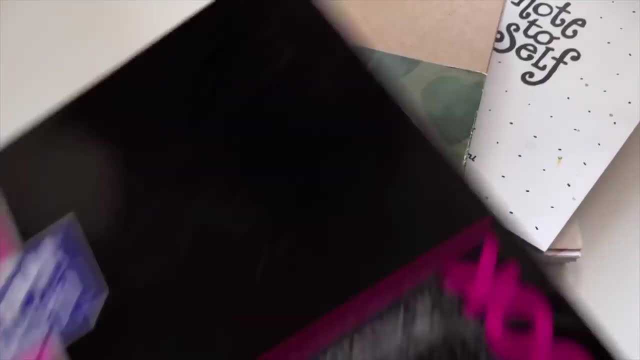 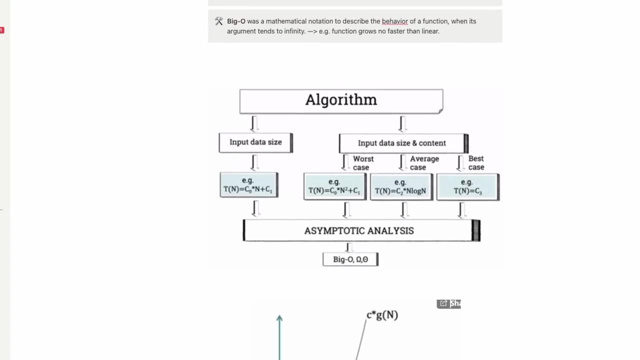 and reinforce that knowledge often enough. In the past I was very keen on keeping physical notes, but now I usually keep digital notes on Notion, just so that I have everything in one system and I can look up things quickly. You can definitely build your own system in many other. 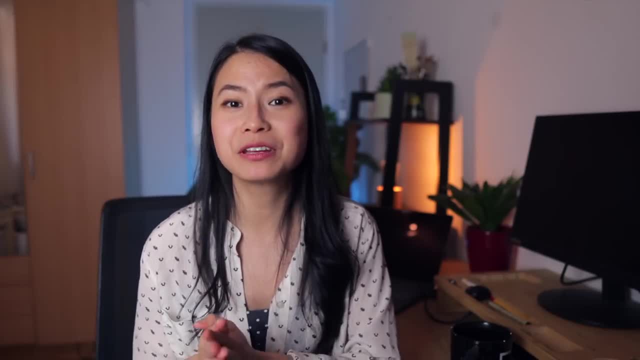 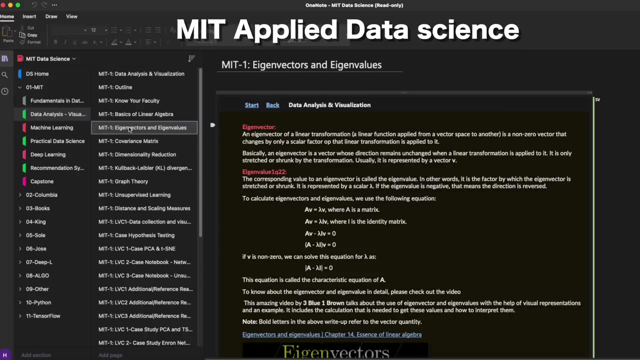 ways. Starfrost, one of the subscribers, reached out to me a few weeks ago and shared with me an amazing system he built in OneNote. He organized everything he learned in the MIT Applied Data Science program in this notebook. It's really an amazing piece of system that makes sure he can. read and write. So if you're interested in learning more about statistics, please subscribe to my YouTube channel. It's really an amazing piece of system that makes sure he can read and write. So if you're interested in learning more about statistics, please subscribe to my YouTube channel. 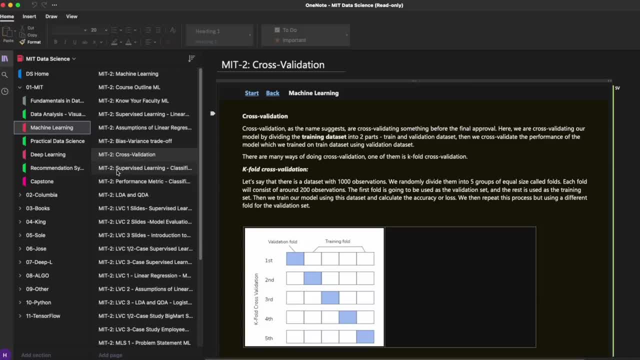 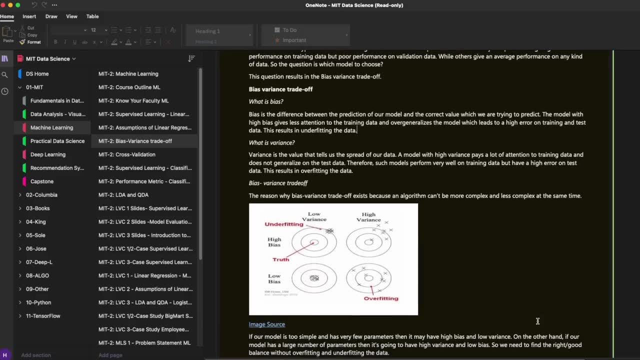 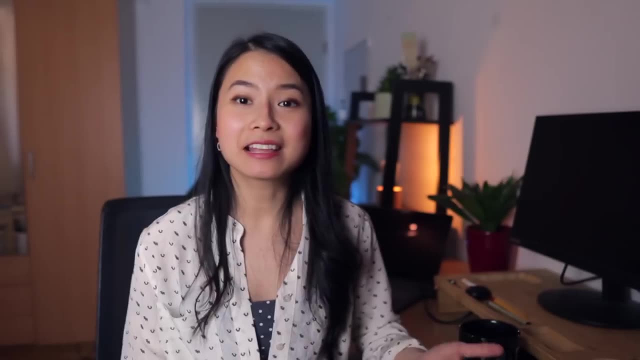 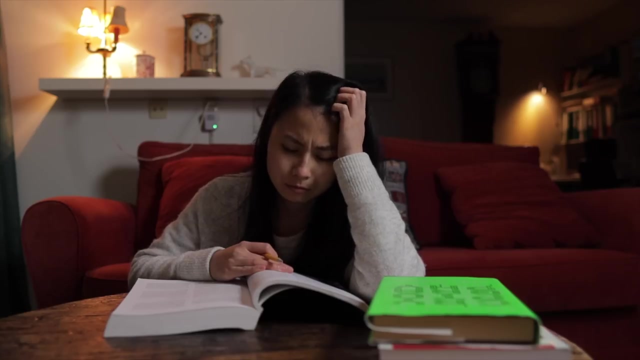 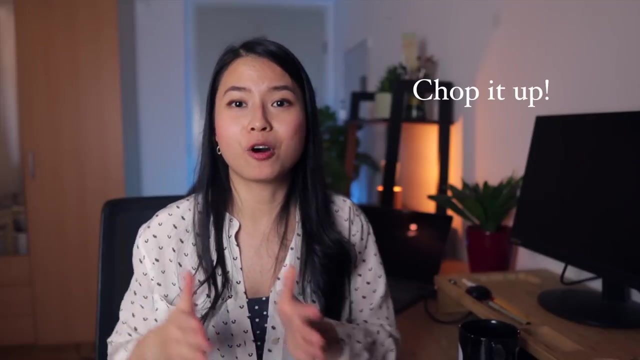 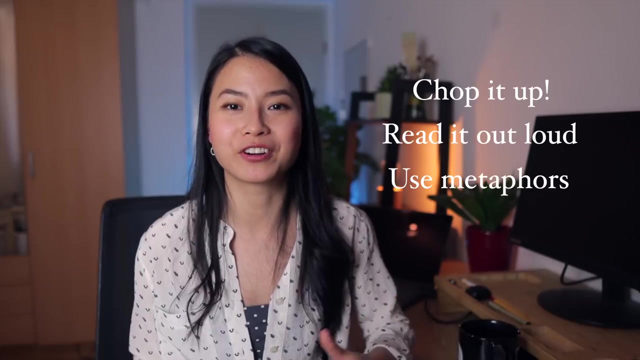 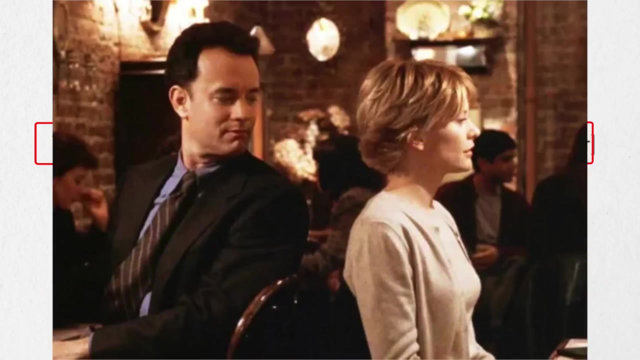 and I'll see you in the next video. Bye for now. find useful to chop the formulas into smaller parts and try to understand each smaller component, and even say it out loud and use metaphors for it. For example, this seemingly complicated function can be broken down into a few parts. And let's put this equation in the dating context. So the 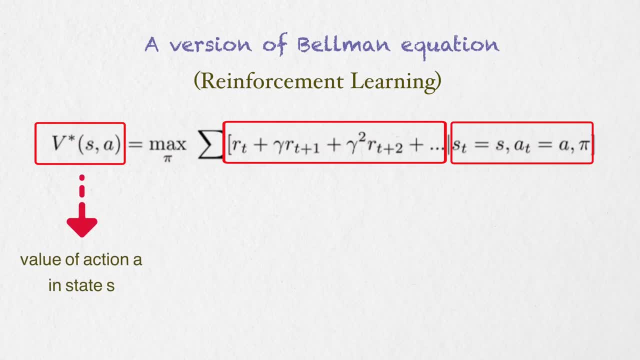 left-hand side basically means the value of action A in state S, Let's say it's the value of calling your date on Friday evening. And this part on the right-hand side basically means the total rewards, including the rewards at the current moment and the total rewards at the current moment. 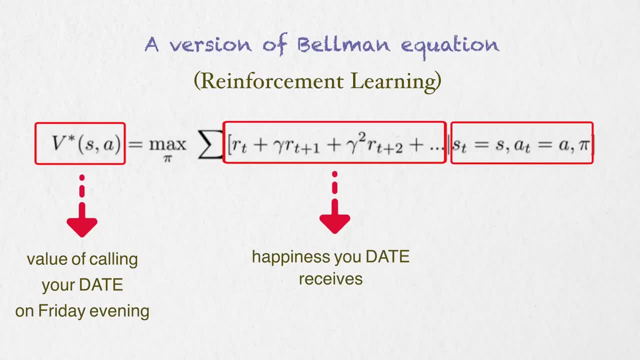 Plus all the discounted future rewards. Or in this case, we can think of it as how much happiness your date will feel right on that Friday and all the following days because you called her. The gamma factor here is smaller than one, meaning that every day, this happiness effect that your 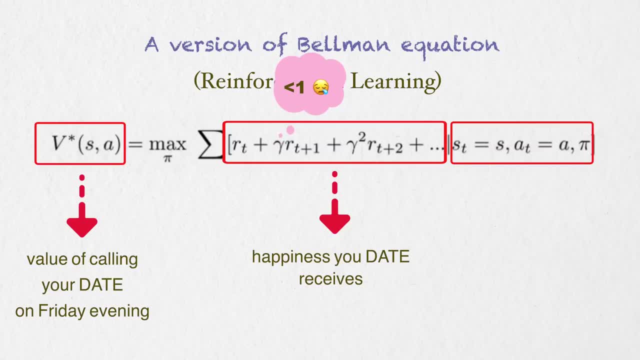 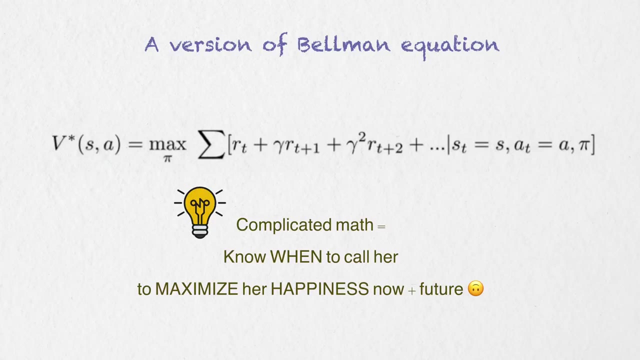 date will experience, will get smaller and smaller because people do forget things. And this part basically means, given your current state and action chosen by the action policy by. So this whole equation in our case can mean finding an action policy, For example, calling your date every X days at a given time, such that 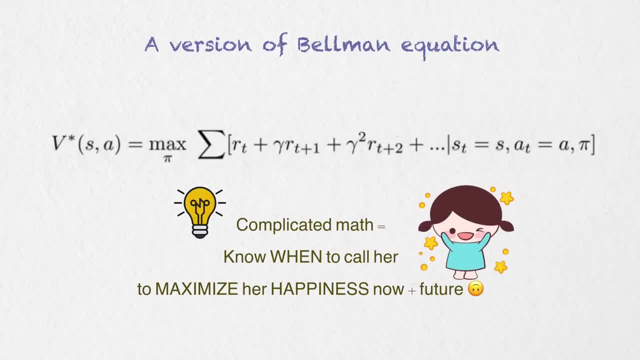 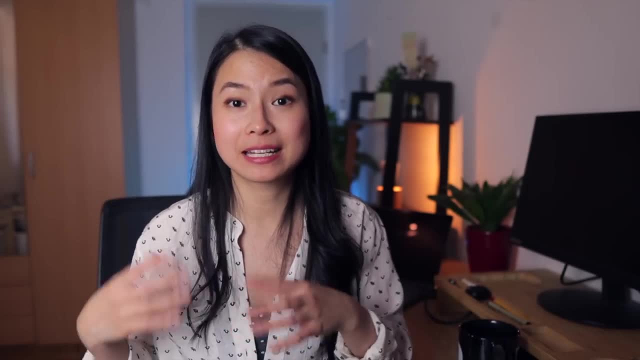 you can maximize the total rewards, which is your date happiness level now and in the future. Well, if so, you're very good at selfishness dates. Breaking things down into smaller parts also makes it easier for us to identify where and why exactly we don't understand something. Maybe it's. 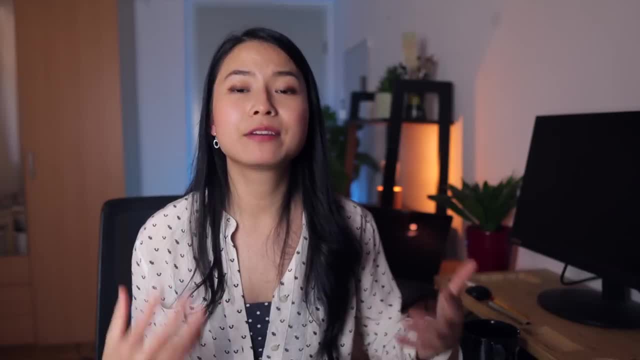 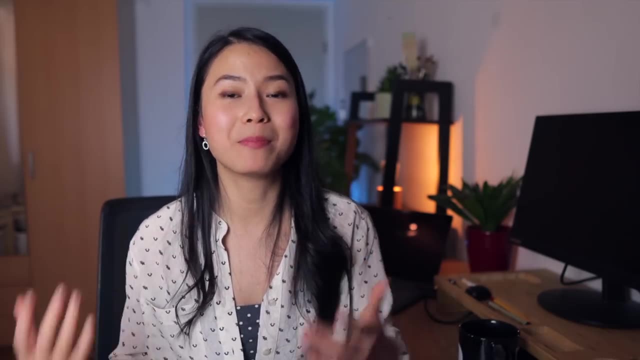 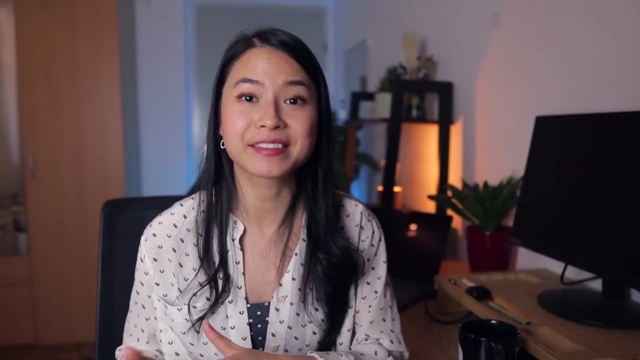 because of some unfamiliar notation or symbol. This will give you some direction to make progress with your understanding and makes the complicated math concepts feel a bit more manageable. Another way of learning I often find extremely useful is to actually code the math formulas in R or Python In the deep learning. 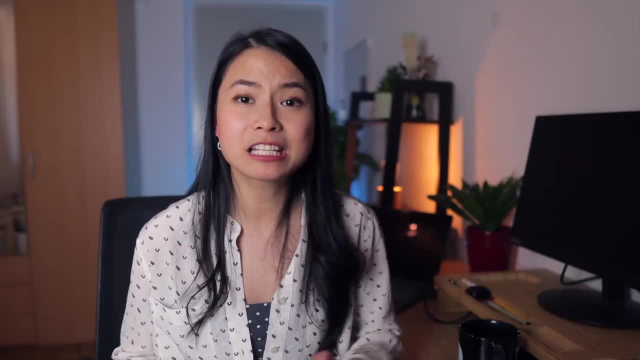 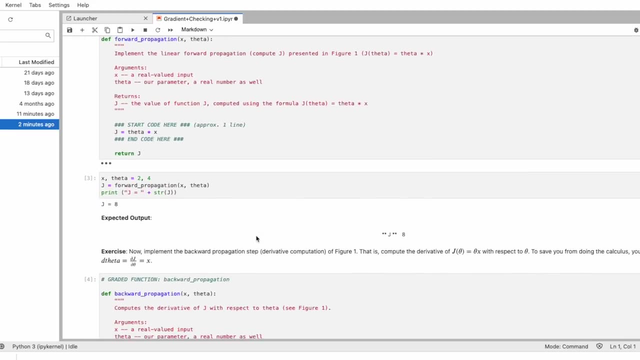 specialization I took on Coursera a while ago. I found it such a great course because you get to code the neural network algorithm from scratch. You get to implement the back prop algorithm yourself- which is probably the hardest part to understand in neural networks- And step by step, 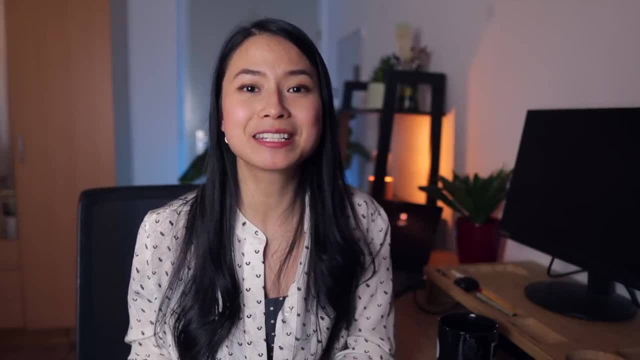 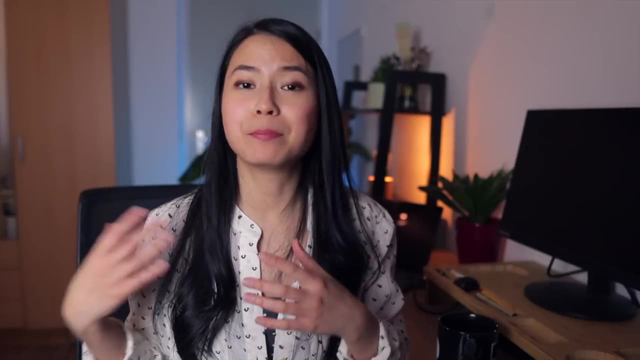 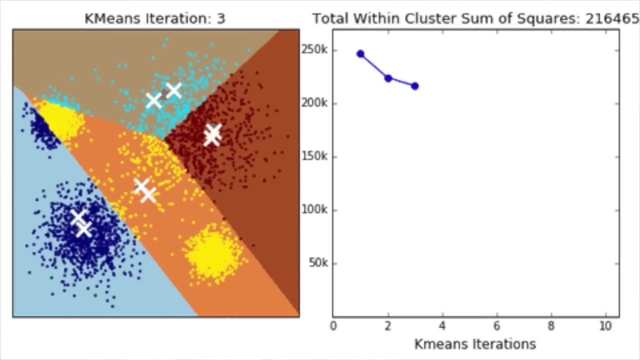 those complicated matrix multiplications and partial derivatives become much more transparent and intuitive because you can code it yourself, And I guess this method can be applied to many different machine learning algorithms. For example, you can try for once coding an algorithm by hand, like k-means, for example, instead of using the out-of-the-box. 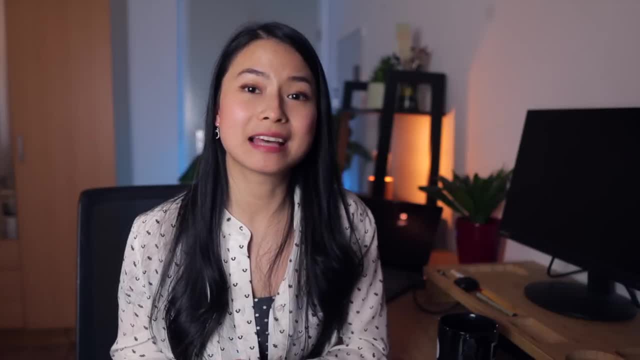 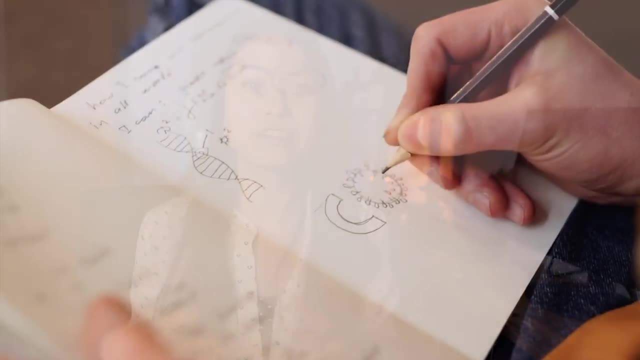 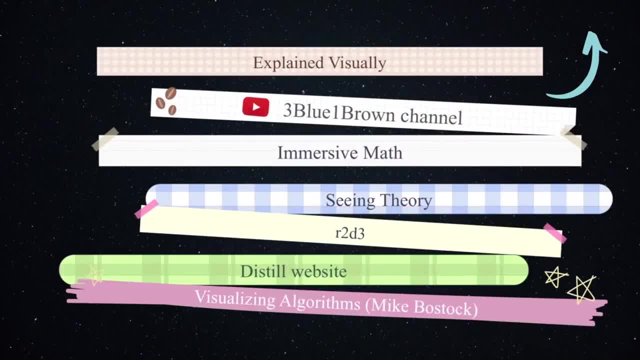 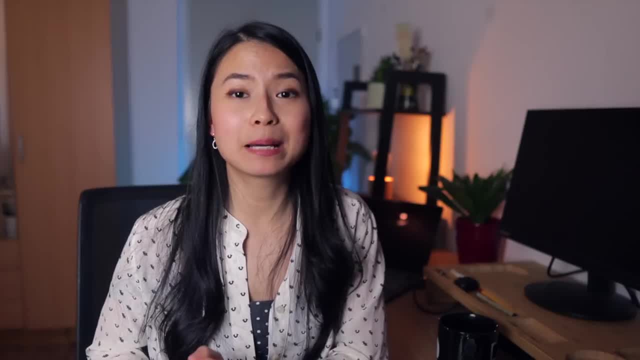 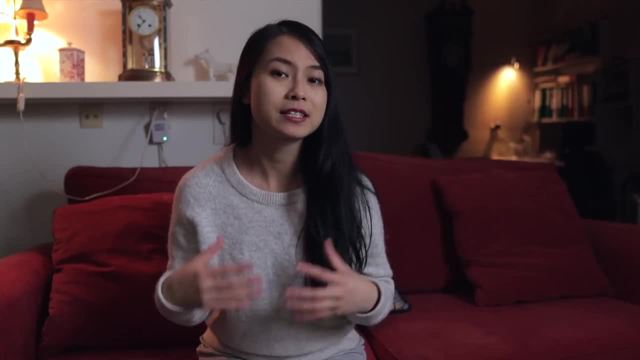 We have interactive books, tools and also YouTube channels like 3Blue1Brown that focus on explaining things with animations and visualization, And so all these abstract concepts become much easier to understand and digest. One of the very common feelings that we face when learning math is the imposter feeling. 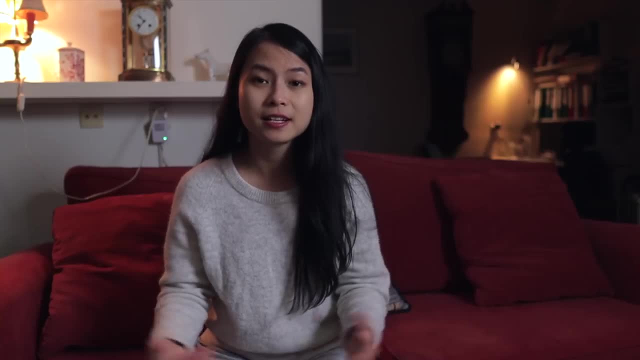 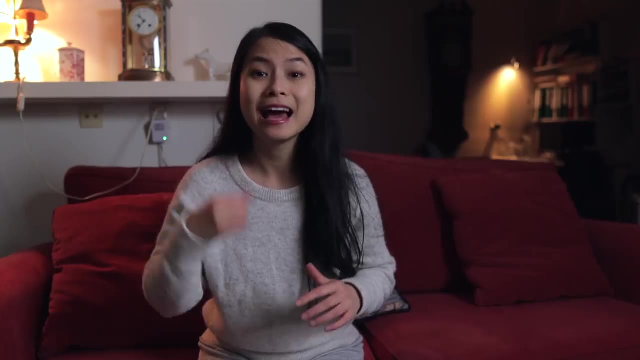 But it is what it is. It's just a feeling. One of the lessons learned for me is when you feel imposter, you don't need to act on it, Just let it pass. But when you feel the motivation, act on it, Keep learning And realize that that feeling probably doesn't have much to. 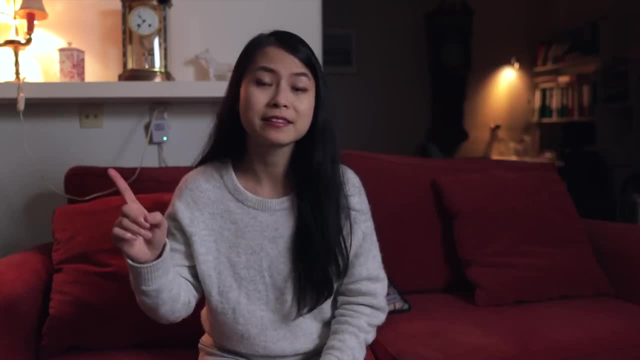 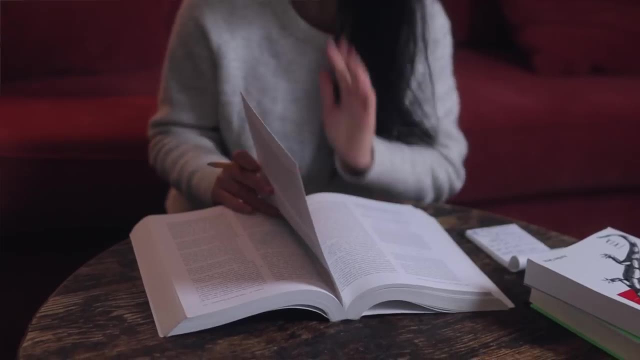 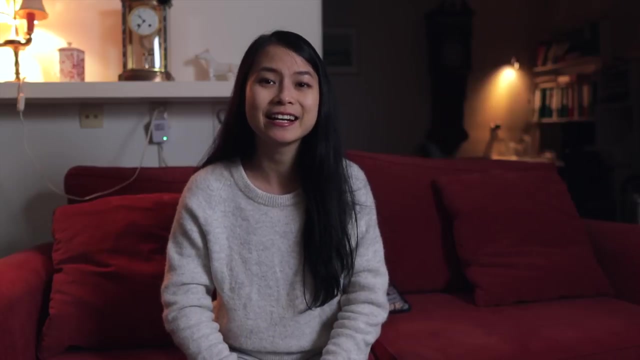 do with your true ability and your knowledge. And also another thing that I learned is that when you don't understand something- for example, if you read a book and it feels like this whole thing is so complicated and you feel like you want to give up and you feel like you're not smart enough to understand it- 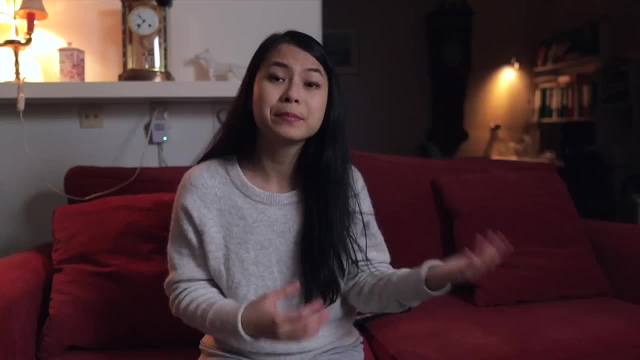 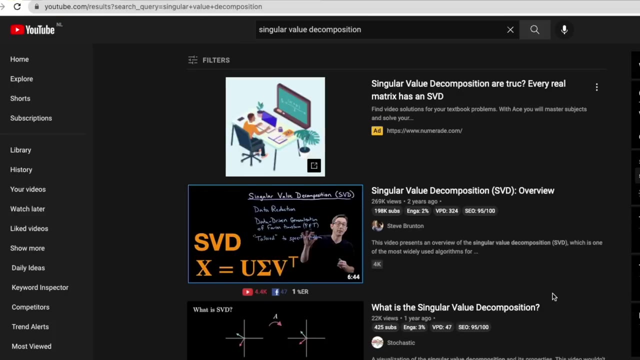 actually, it's probably not all your fault. It could also well be that that book doesn't explain well enough that concept. I would go on YouTube, on Google, on Google, Play, Google, to find a better explanation, a better presentation of what I've tried to learn. 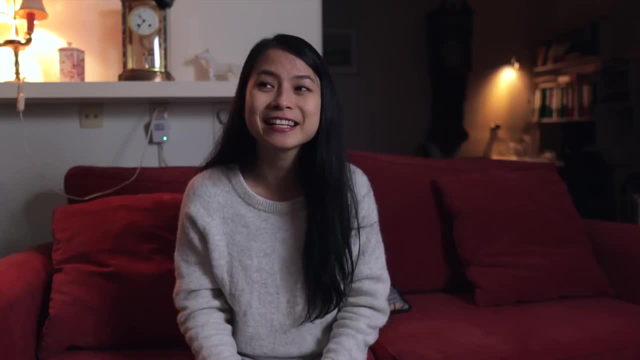 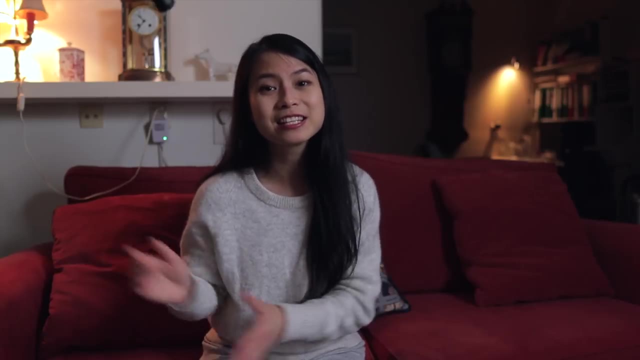 And most of the time, there is a better explanation elsewhere on the internet. I hope you enjoyed these tips and don't forget to check out this video about how much statistics you need to know for data analysis. With that, I'll see you in the next video. Bye, bye.